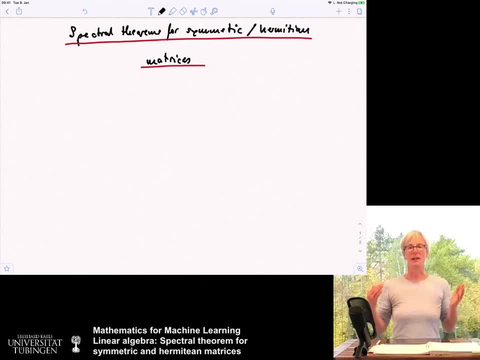 are real, And the other thing that we have seen is that eigenvalues, or eigenvectors corresponding to different eigenvalues, are orthogonal to each other. And this, in fact, is not only true- the second part- for complex-valued vector spaces, but also for real vector spaces, And 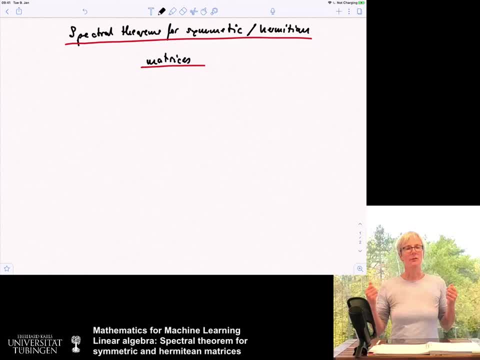 we have already seen that if you have a symmetric matrix, it has at least one eigenvalue and one eigenvector. then, of course, And now we want to prove what is known as the spectral theorem for symmetric matrices. This is really the most important theorem. 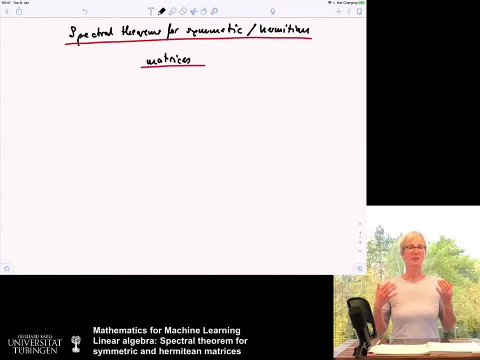 regarding the spectrum of symmetric matrices. This is the most important theorem regarding symmetric matrices and this is going to save our lives in machine learning, because without that theorem we would be doomed Like most of the methods, or at least half of the methods I know probably would break down if that theorem wouldn't exist. So let me try to write down. 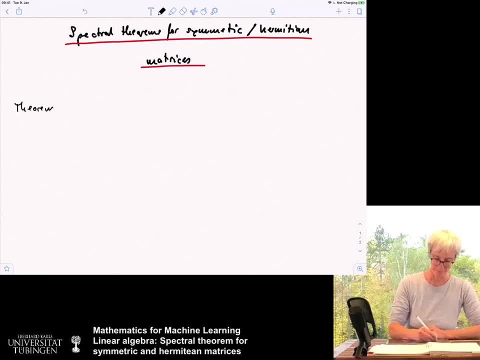 the theorem A symmetric matrix A that lives in Rn times N- so we are over the real numbers in this case- is orthogonally diagonalisable. Othogonally diagonalisable. You can practice that to say that yourselves. 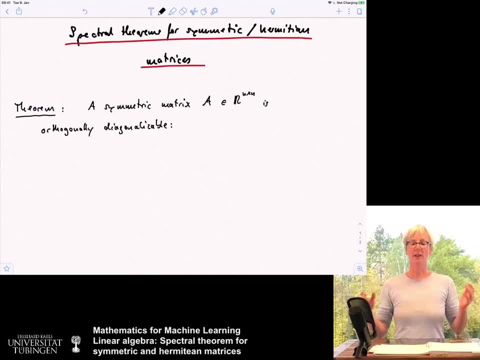 What does it mean? There exists a matrix, there exists a base. it's such. if I don't close the windows, I'm going to suffocate in this room. it's gonna be extremely hot if I keep the window open. there's this: 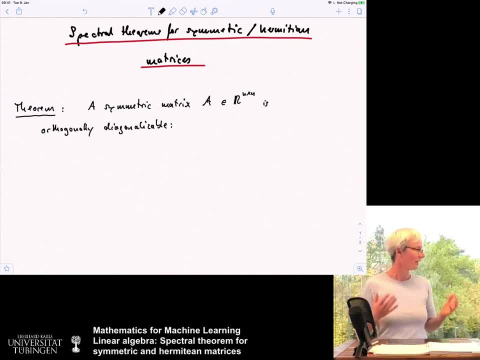 truck driving back and forth all day, and now I'm going to close the window. okay, there we go. a symmetric matrix is orthogonally diagonalizable. what does it mean? there exists a basis and an orthogonal basis, and, in particular, such that the matrix that represents this linear operator consists just of is in diagonal form, and all the basis. 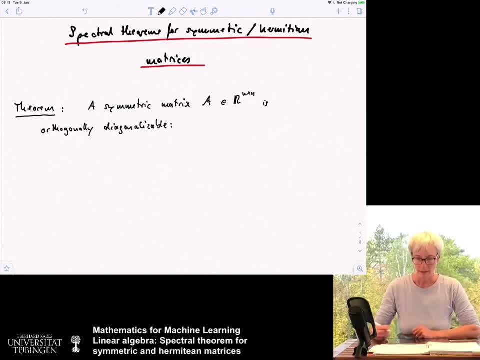 transformations are also really nice, so let me just write it down. so there exists an orthogonal, and there exists an orthogonal matrix Q in R n times n and a diagonal matrix, D, also in R n times n, such that we have a can be written as Q, D, Q transposed okay, so D is the diagonal matrix. we have this. 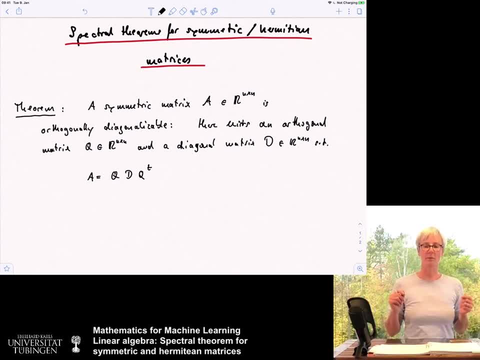 orthogonal matrix Q, which does the basis transformation, observe that the inverse of this orthogonal matrix is Q transpose. so I don't need to write Q minus 1 here Q to the power of minus 1, here Q inverse. but Q transpose is fine. and so what I'm going to do is I'm going to write this diagonal matrix, Q transpose, and I'm going to 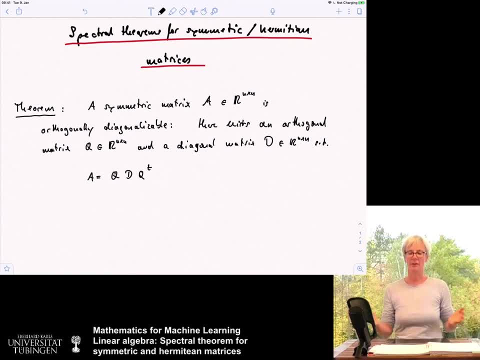 write a diagonal matrix, Q transpose, but Q transpose is fine, and so what I'm going to do is I'm going to write this diagonal matrix, Q transpose, and I'm going to original basis was I can transform it to this other basis such that I have this problem and, if you want, I just write down another way of writing this. 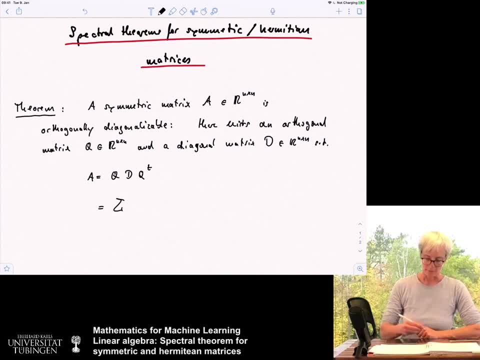 the same result you can write- let's just make a nicer some time. it is: the sum of I equals 1 to n. lambda I, Q, I, Q. I transpose, which is 3 times P by I, and where lambda i are the eigenvalues and qi are the eigenvectors of this matrix. 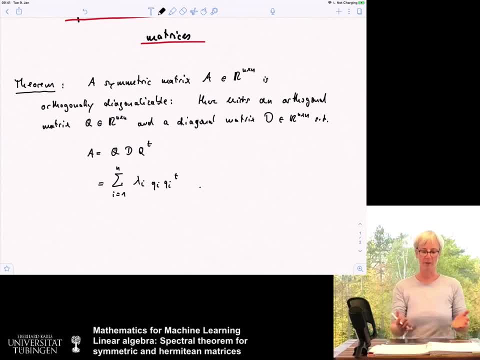 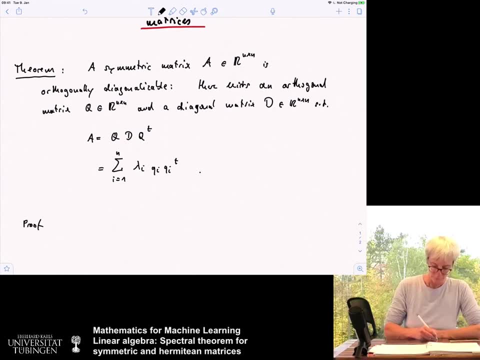 So this is the real spectral theorem. It looks pretty harmless, but this is what it is. Now let us prove that theorem Proof. And again, this is just going to be a sketch, but I want to give you the glimpse how it works. This is a proof that goes by induction. 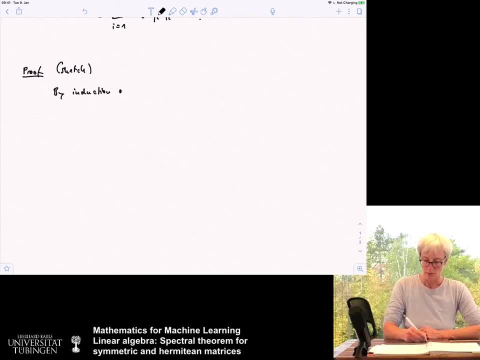 By induction on n, which is the dimension of the vector space. I mean this whole thing operates on a finite dimensional vector space. Observe that on infinite dimensional spaces these kind of spectral theorems are not as simple as here, Because a spectrum can be something that's much more complicated in an infinite 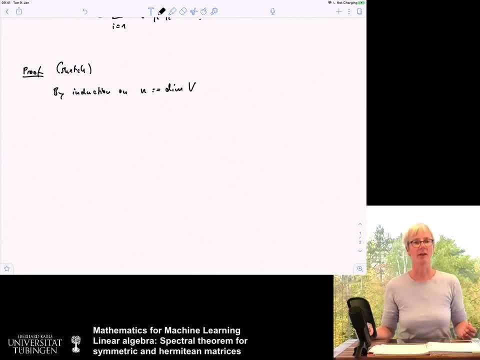 dimensional space, because a spectral not only consists of eigenvalues, like an element in a spectrald doesn't necessarily mean that there is an eigenvector, because in a finite dimensional space. What is so nice about finite dimensional spaces is that mapping is invertible if, and only if, it's not injactive. 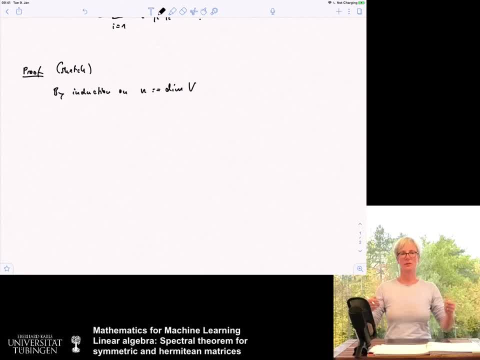 It's not alright if it's not not too injectative and at the same time not surjective. so these things are equivalent In an infinite dimensional space. this goes wrong. So you could have different reasons why something is not invertible. It could be either because the thing is not injective. 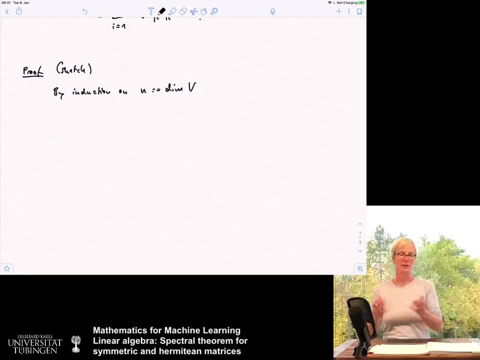 this leads to an eigenvector, or because it's not surjective, and that leads to something else And that makes it much more complicated. But here we are in a really nice finite dimensional space. So sorry, I lost trace a bit. 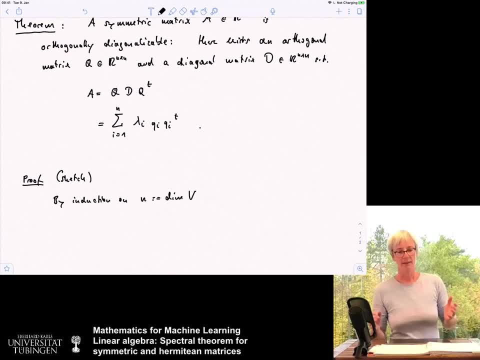 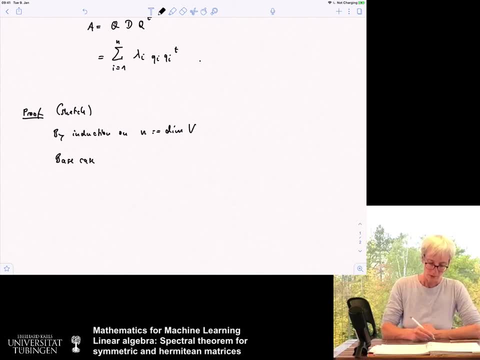 We want to prove that real-valued spectral theorem by induction. and n is the dimension of the vector space. So how does a proof by induction work? We first of all start with the base case. In our case this is n equals 1.. 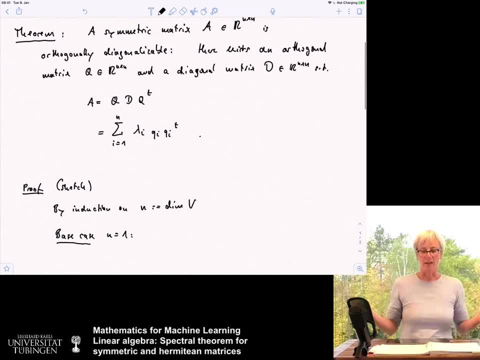 And for n equals 1, the theorem is pretty clear, because then, like, a symmetric matrix is just a linear number, it's just a number and everything is sort of here. we just multiply by a number and then everything here is sort of trivial. 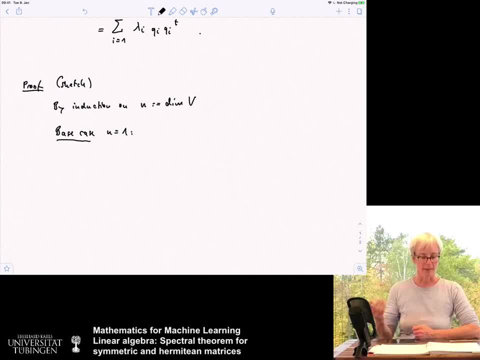 So that's not the interesting case. What is interesting is the inductive step. Inductive step that takes us from hold it here. how would I do it? n minus 1 to n. Okay, so we start with. we now want to prove. 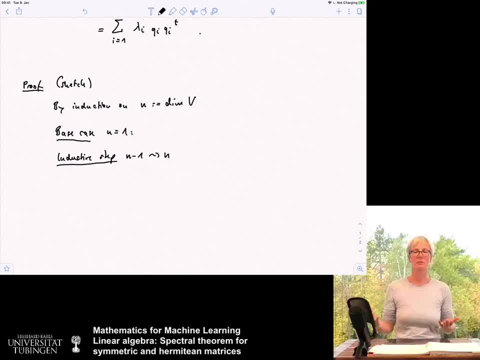 we have already proved for n minus 1 that this statement is true, and now we want to prove it for n. So we start with observing that, because a is symmetric by the previous proposition that we have seen, there exists at least one eigenvalue and eigenvector of a. 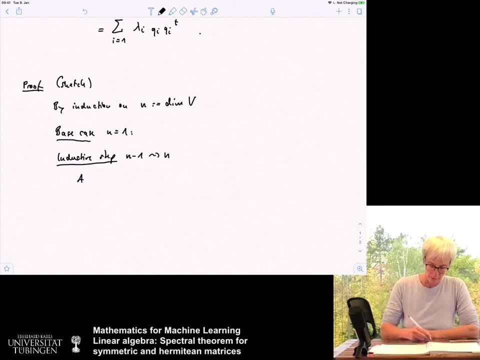 This is something that we have already done. This is something that we have already proved. So a is symmetric. This implies a has at least one eigenvector, which is called u, And with the outlaws of generality, we assume that the norm of u is 1,. 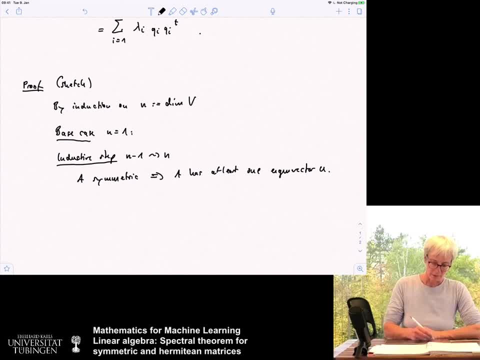 but that's maybe not so important for now. And now we can define the subspace that is spanned by u. So we define: u is the span of this eigenvector, lowercase u, And the subspace u is invariant under a. 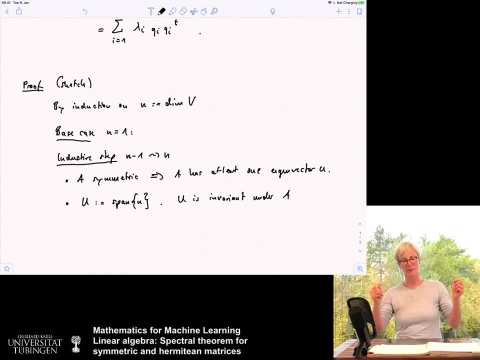 Invariant means if I apply a, then I end up like if I start with a vector in u and apply a, then I end up again with a vector in u. This is a one-dimensional space consisting of of an eigenvector. 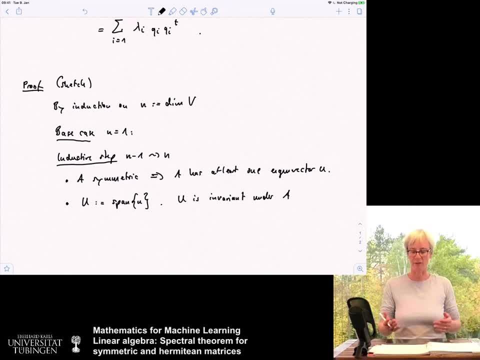 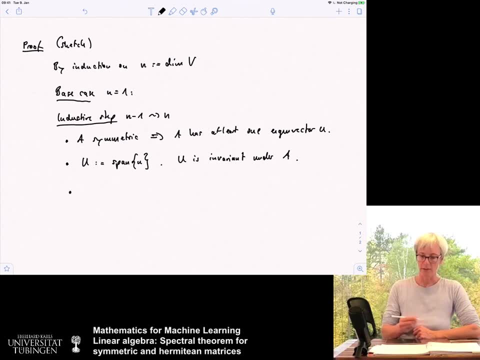 So this is true. This is sort of the more or less very definition of an eigenvector. Okay, So far so good, So nothing really complicated yet. And now we consider the orthogonal complement of u. Consider the orthogonal complement of u. 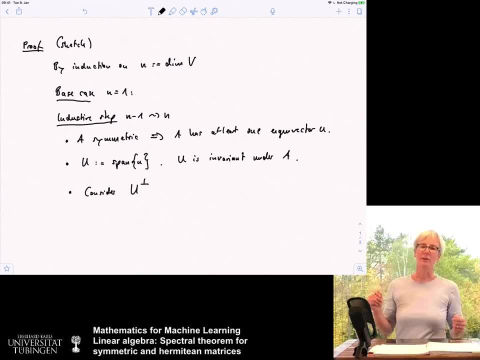 And now we consider the restriction of the operator a on this orthogonal complement. Consider u And the restriction, the restriction of a to u-orthogonal. So we simply want to apply a to vectors that come from this u-orthogonal. Now the point is on this subspace: 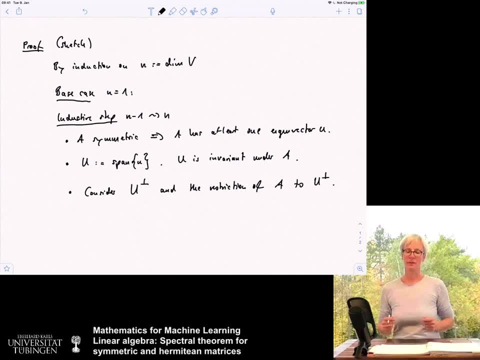 this restricted operator is again a self-adjoint operator And this is sort of the key ingredient here On u-orthogonal a is again a self-adjoint, so symmetric. if sorry, I could also write, maybe I write symmetric operator. 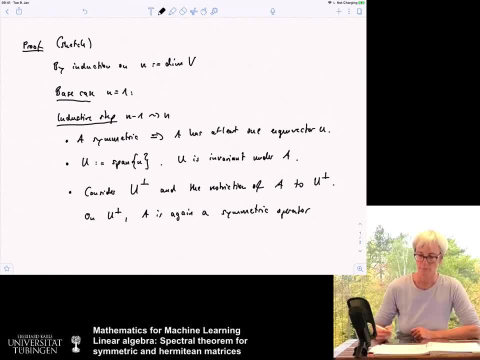 And it now operates on u-orthogonal. So this is a self-adjoint operator And it now operates on u-orthogonal And it now operates on a space of dimension n-1.. And dimension of u-orthogonal is n-1.. 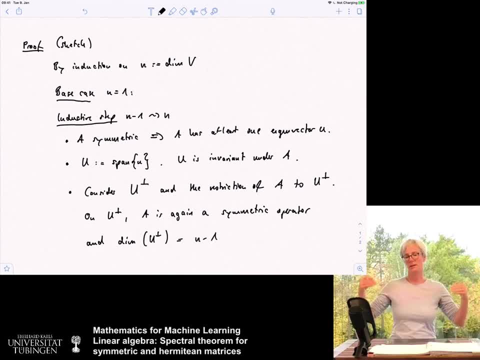 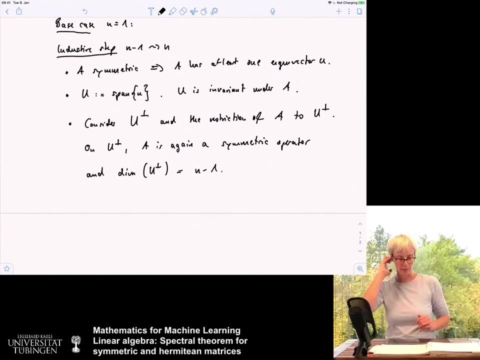 The latter case is clear because I mean, we, like the whole space is a direct sum of u and u-complement. u has dimension 1, so the complement has to have dimension n-1, so that's clear. But there is some work that you need to invest to see that a is again a symmetric operator. 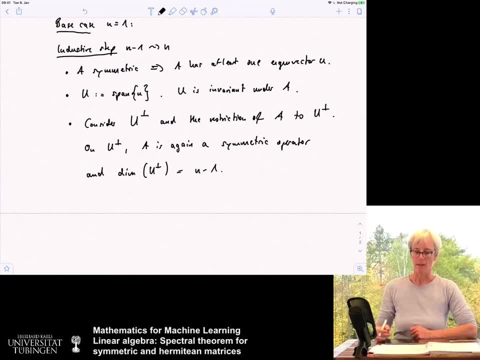 So I'm not going to write this out here, I just want to give you the sketch. But because we know that we can now use the induction hypothesis And then essentially we're done, Now apply the induction hypothesis on this lower dimensional space, on this space. 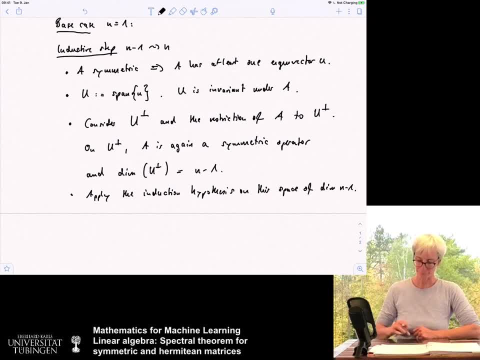 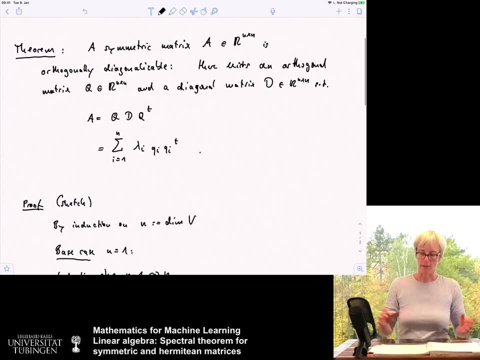 of dimension n-1.. And then essentially the induction hypothesis. then essentially you're done. The induction hypothesis now tells you that on this lower dimensional space you have this decomposition, you have these eigenvectors, and now you can take the eigenvectors of this lower dimensional space. 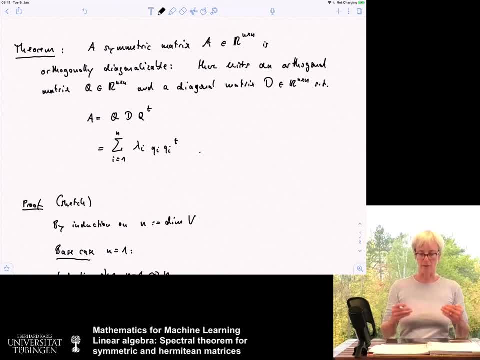 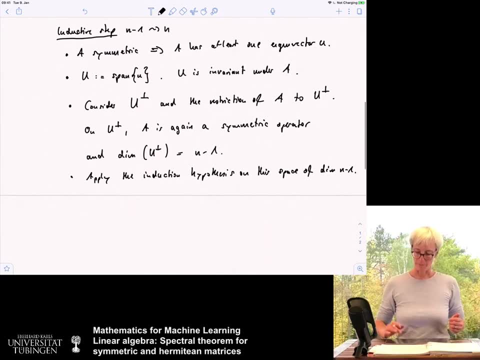 and there and add this last eigenvector u1 that we had constructed in the very beginning, and then we have a basis of the original space, which does the job. I simply write: does the job. Of course, if you want to write it down properly, this is probably another page of writing down why it really does the job. 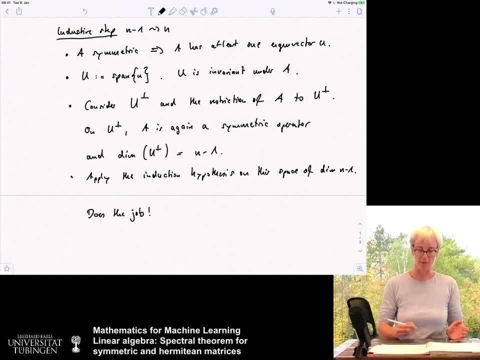 But I think the intuition is clear and I don't want to spend that one page. So this is the proof sketch, at least for the real-valued spectral theorem, And I want to stress that, And I want to stress again that this is really one of the most special theorems. 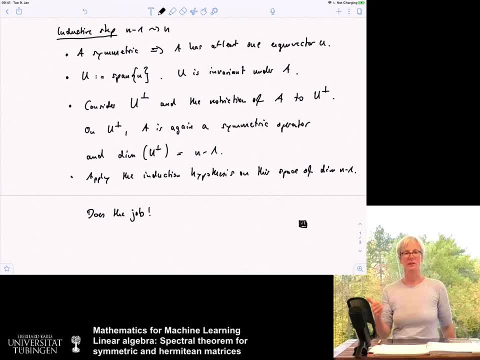 in particular also for machine learning. So what it says is, first of all, the eigenvalues exist. That's the first property. They're real-valued. I mean, okay, if we talk about complex eigenvalues they would exist anyways, but they exist. 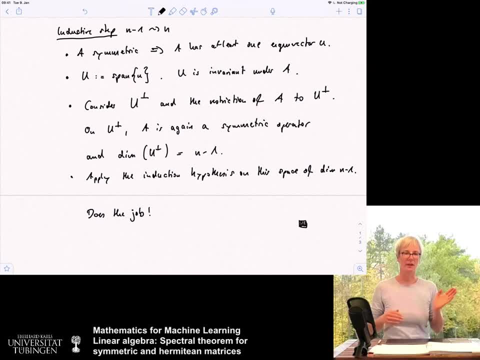 They're real-valued And the eigenvectors. if the eigenvalues are different, the eigenvectors are orthogonal to each other. This is really an extraordinary set of properties And in machine learning we use that all of the time. 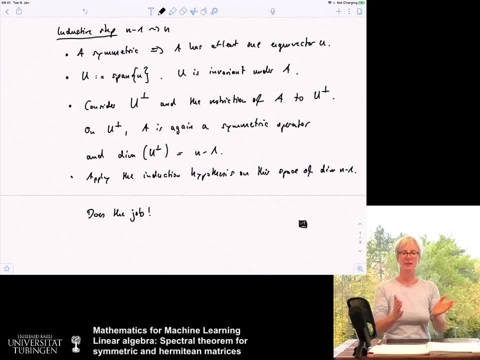 So when we do principal component analysis, it's applying this particular theorem. It's really and when I learned it as an undergrad. so it took me two years of being a machine learning PhD student until I realized that the theorem that in German has a very obscure name. 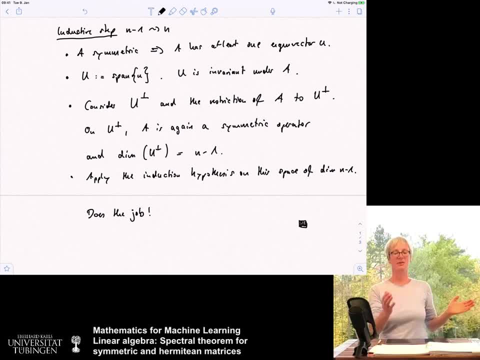 and in mathematics people call it the Haupt-Achsen-Transformations-Theorem or something like that. Nobody ever gave me the intuition, and it took me a long time until I realized that this thing that I learned in my education- my undergrad in math- is: what is PCA in machine learning? 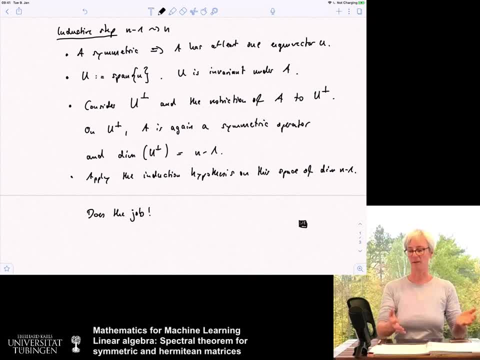 So this really is PCA or SVD if you want, but let's call it PCA here, And also whenever we have similarity matrices or kernel matrices. this is going to be one of the key objects that we're going to operate, at least in standard machine learning outside of deep networks. 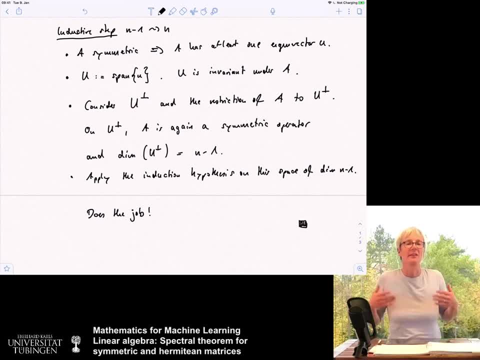 then you always have symmetric matrices And it's hard to conceive. It's hard to conceive any construction in machine learning that uses these kinds of symmetric matrices and uses linear algebra but doesn't make use of this particular theorem. So it's really one of the most important theorems that exists out there. 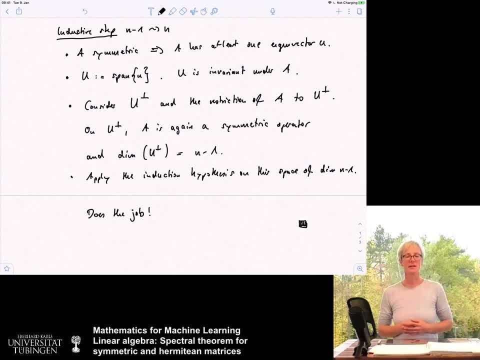 And if you happen to be in my next term lecture on statistics in machine learning, and if we happen to be able to do that lecture not online but in classroom. whenever we see a symmetric matrix, I'm going to ask you: what is the property of this matrix? 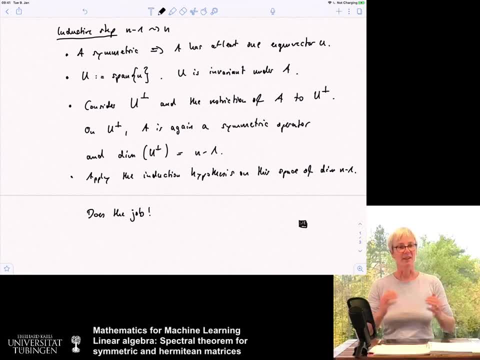 And you're going to answer. it has a basis of eigenvectors which are orthogonal to each other and the eigenvalues are real valued. It is really. this is something you need to know and you're not going to survive machine learning if you don't know that. 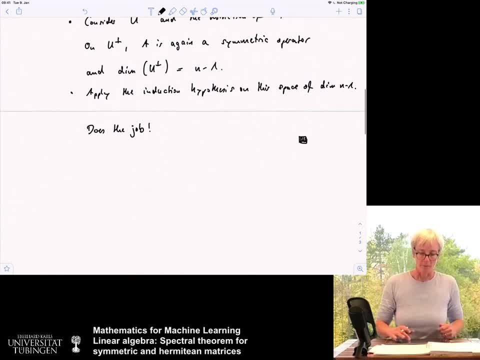 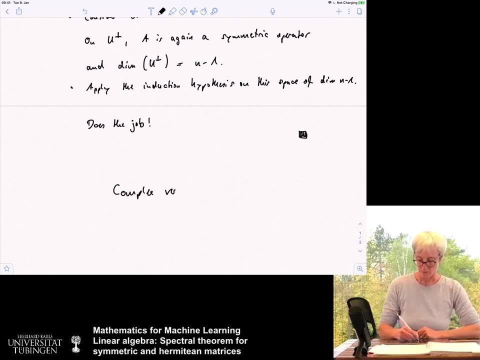 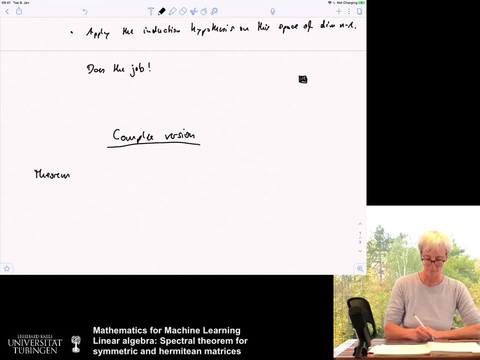 Now there also exists a complex, valued version of that theorem, which is now not so surprising anymore. I just write it down, the complex version of that spectral theorem. So theorem: now we have a Hermitian matrix, Hermitian matrix A in our C? n times n.